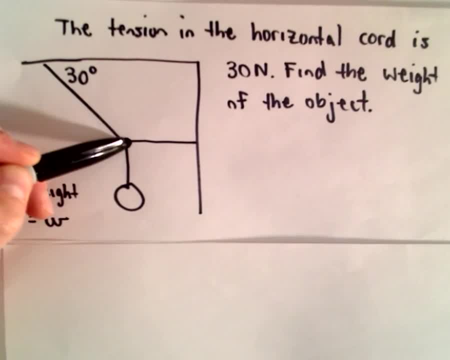 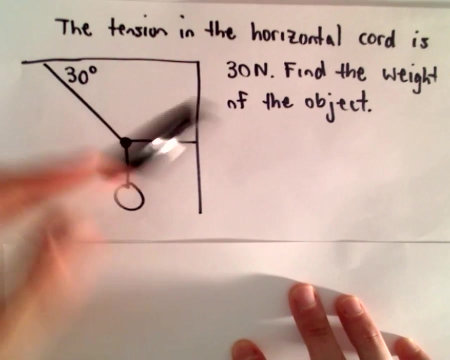 So we've got some object hanging from a cord and there's a knot that connects these three cords in general. So we've got the weight of the object. We've got a cord that connects it horizontally to the wall. We're told that the tension in that horizontal cord is 30 newtons- and this other cord that's connecting it to the ceiling. 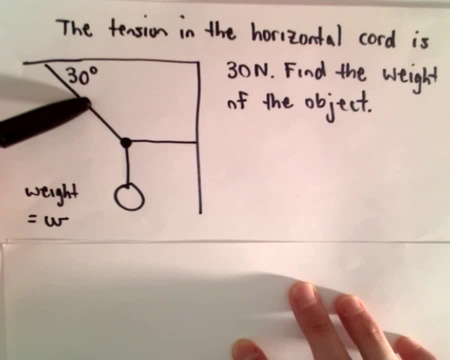 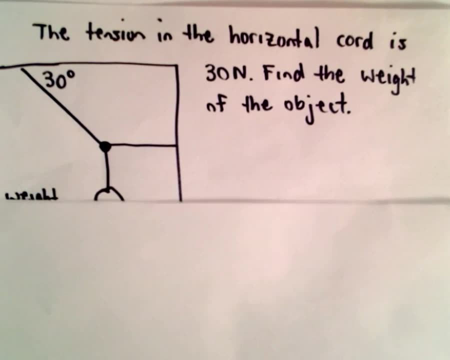 we don't know its tension, but we know it makes an angle of 30 degrees, And from that information we want to find the weight of the object. Okay, so what I'm going to do is I'm going to make what's called a free-body diagram. 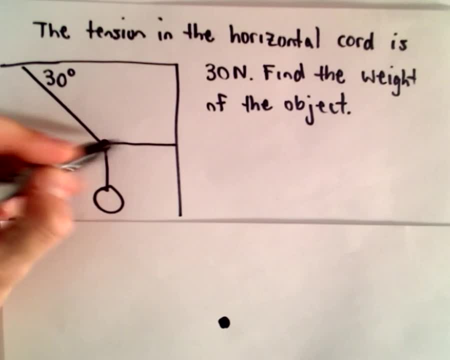 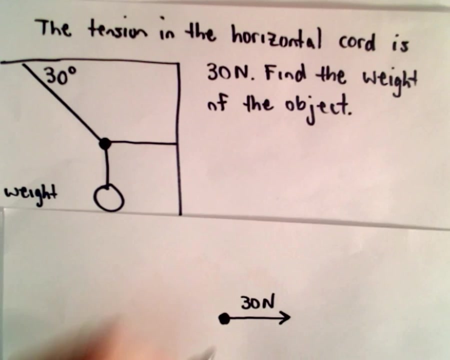 So I'm going to think about this knot that connects the three cords, And what I'm going to do is just label all the vectors, All the vectors that are acting on that knot. Okay, so I know that there's a horizontal vector, a horizontal force here of 30 newtons that's given to us. 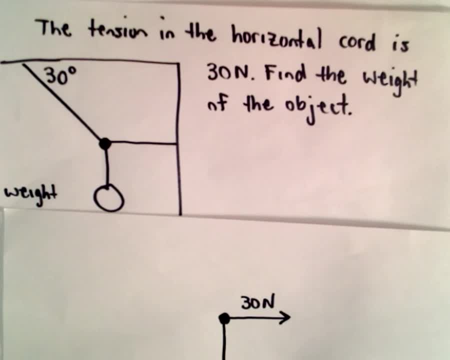 There's also a vector that's pulling it down. Okay, so there's a vector acting in the downward direction here, And the force or the tension- maybe I'll call that cord T1, the tension that would be acting on that cord would simply be the weight of the object. 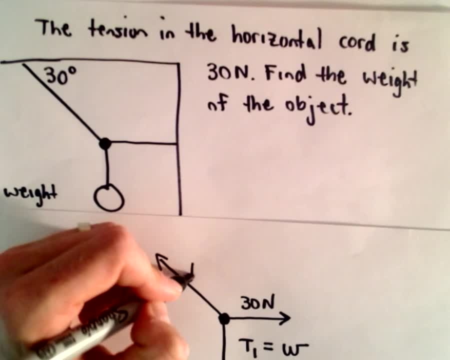 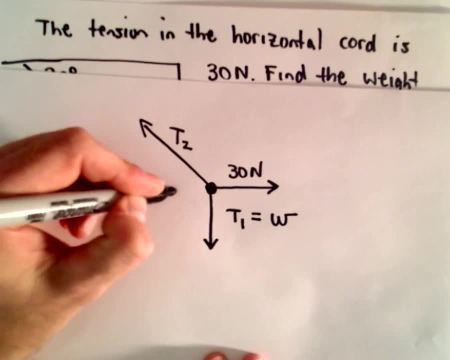 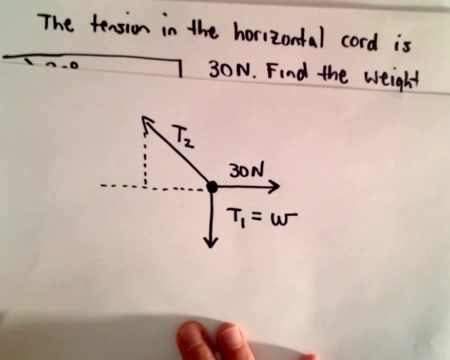 Now we also have this other cord. I don't know its tension. Let me maybe just label that as T2.. What I'm going to do is I'm going to break down this left side into its horizontal and its vertical components. Alrighty, so again, to do this, we can just use a little bit of basic trigonometry. 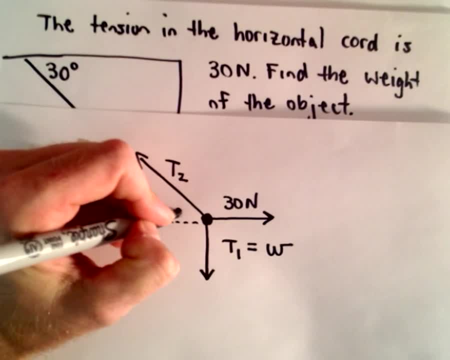 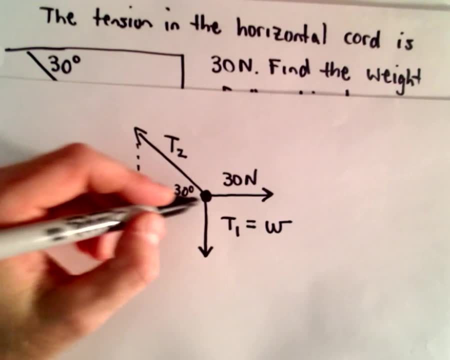 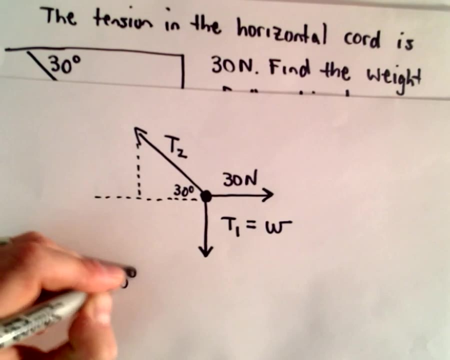 This angle is 30 degrees, So we can conclude that this is also 30 degrees. just basic geometry there. So to break it down into its horizontal and vertical components, we're just using sine and cosine. So just to refresh you real quick, hey, sine of 30 degrees. 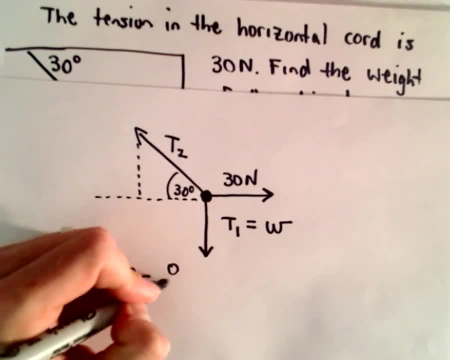 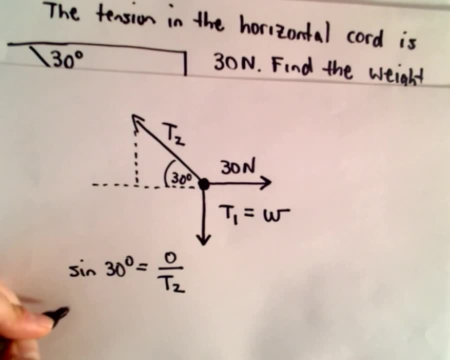 So sine of 30 degrees. that's the ratio of the opposite side to the hypotenuse. The hypotenuse has some tension. We're calling it T2.. So it says the opposite side will be T2 times sine of 30 degrees. 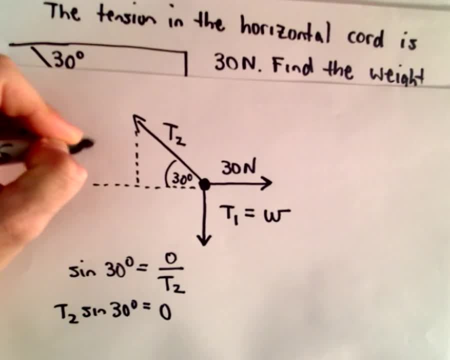 That's going to be the vertical component. So T2 times sine of 30 degrees. And likewise, to get the horizontal component, instead of using sine we'll use cosine. We have T2 times cosine of 30 degrees. That's going to be the horizontal component. 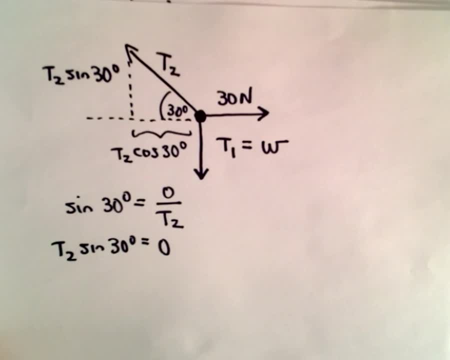 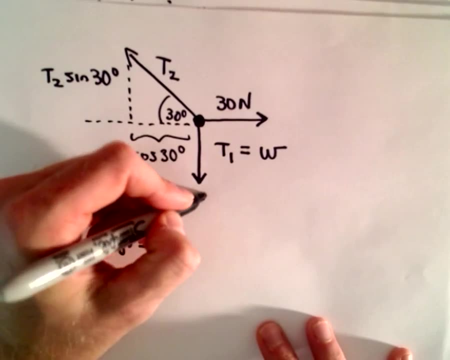 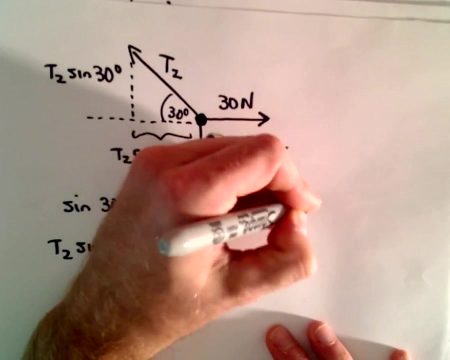 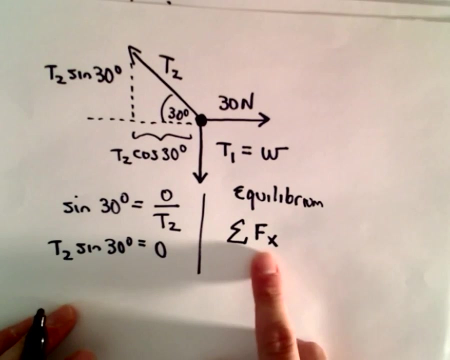 So this is a very common thing with these equilibrium problems, breaking everything down into horizontal and vertical components, So something you'll do all the time. Now the observation is, since everything's in equilibrium, that says, if we sum up the horizontal forces or the forces in the x direction, 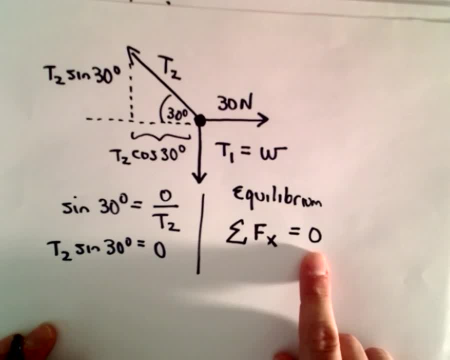 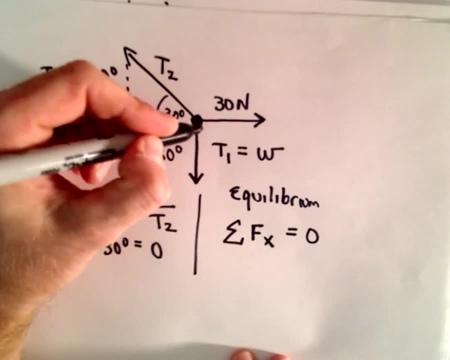 it says: if we sum up those forces, we're going to get 0 again, because it's in equilibrium If the sum was not 0, it would mean that you know the knot here is getting pulled either to the left or to the right. 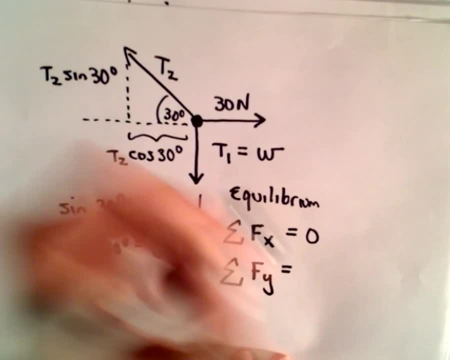 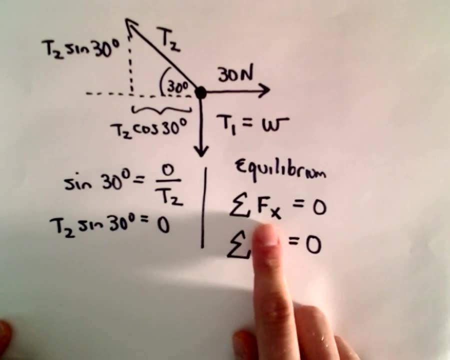 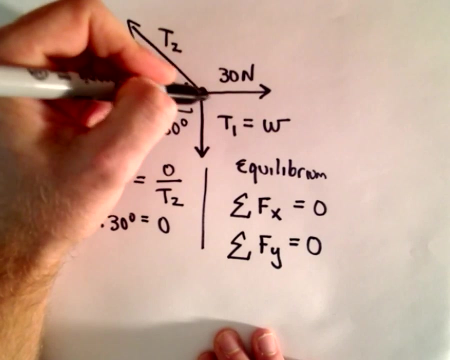 Likewise, if we sum up the forces in the y direction, in the vertical direction, that's also going to have to equal 0.. Okay so if we sum up the forces in the x direction, Okay so, in the x direction, and maybe I'll just make to the right positive, since we normally that's kind of the typical convention. 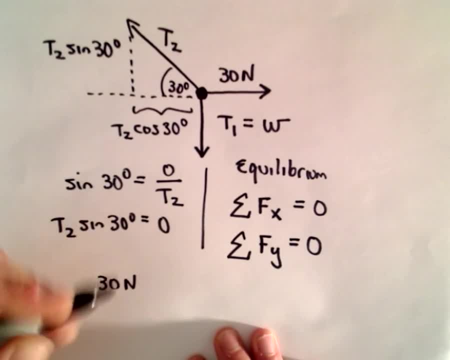 So, to the right, we've got a force of 30 newtons. Well, to the left, we have a force. We've had this T2 component, We've had this T2 cosine- 30 degrees. But since it's pointing to the left, we're going to make that negative. 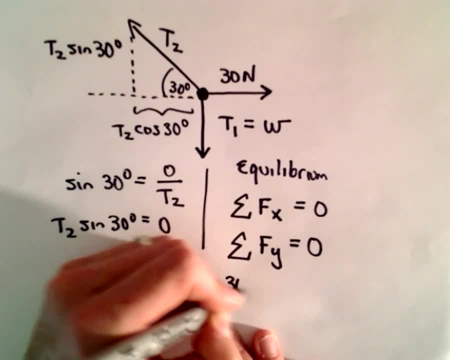 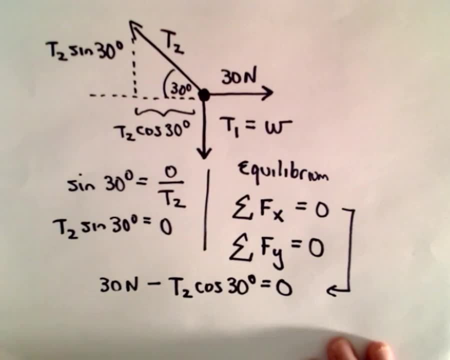 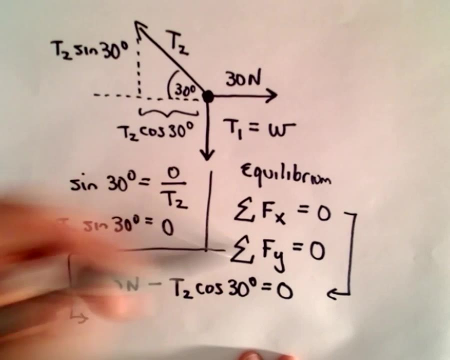 So we have T2 times cosine of 30 degrees, That's going to equal 0.. So that's our equation from our first observation here, And then if we sum up the forces in the vertical direction, that's also going to be 0.. 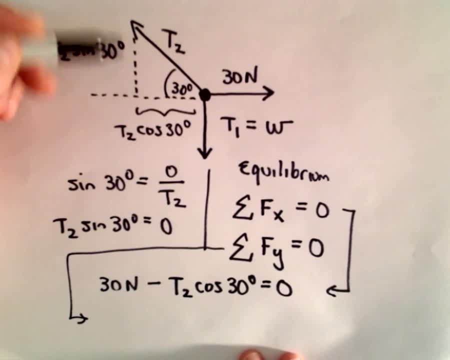 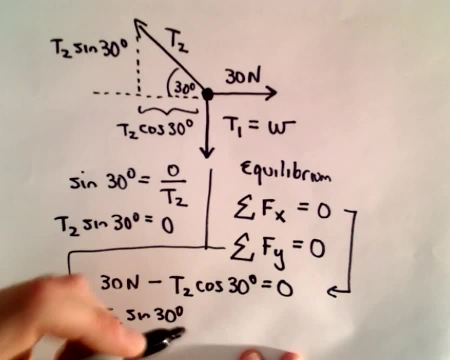 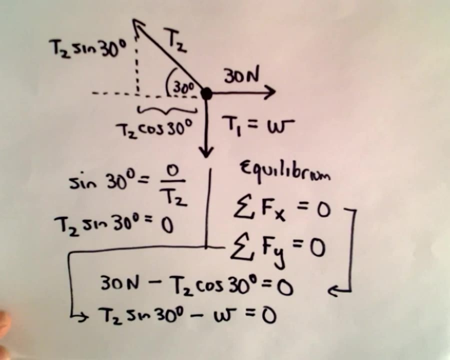 So again we'll just make you know: upwards positive. So in this case we have T2 times sine of 30 degrees And in this case we would have to subtract away W And again that's going to equal 0.. 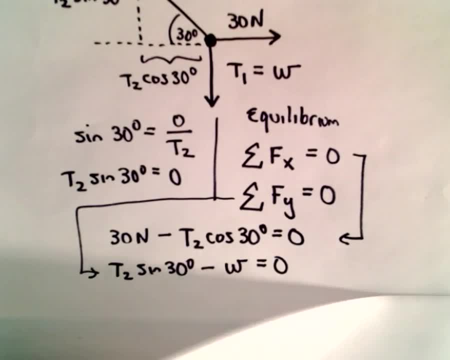 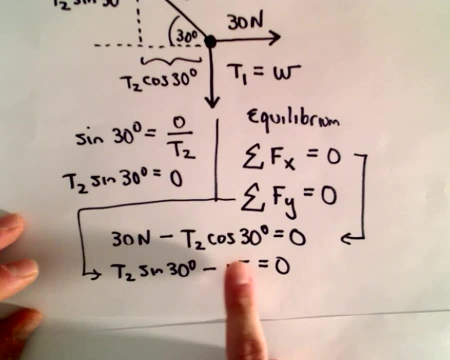 So in this case, all we have to do now is just solve. So I'm going to solve again. we're trying to eventually solve for W. Well, I could solve for W if I knew T2.. Well, I can figure out T2 for my first equation.